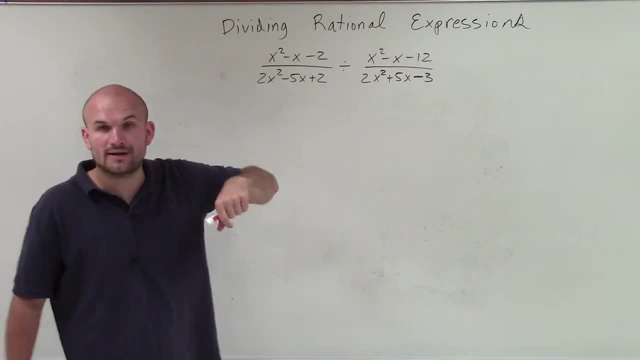 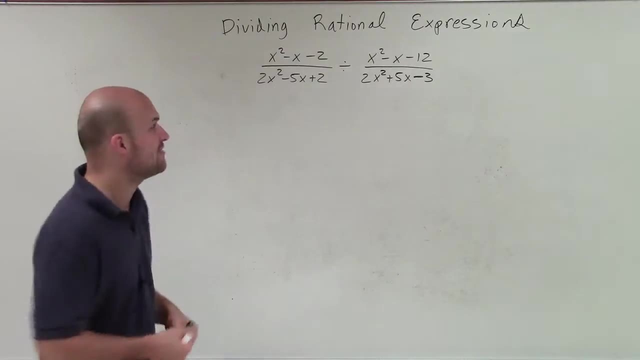 are going to be a little bit more difficult because our a is not equal to 1.. So, rather than going through it step by step, I am going to explain how I'm going to do it, but I am going to do more of a quicker factoring way. So, anyways, our dividend. we're always just 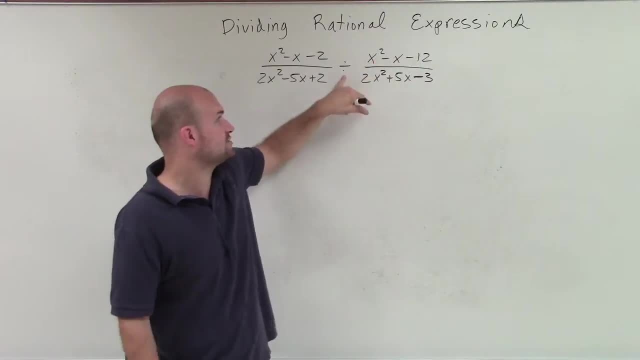 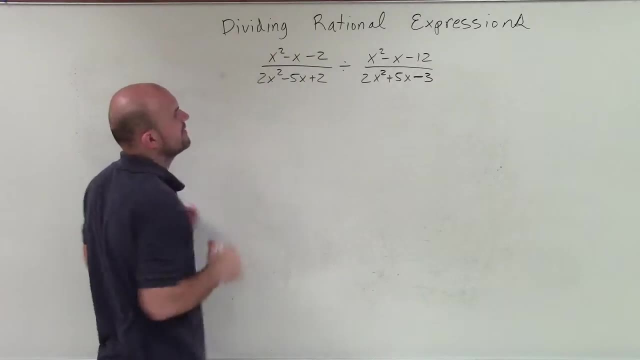 going to simplify this and then, when we simplify this, we're going to make it a little bit easier. We're going to make sure we change this to a multiplication problem and reciprocate, All right. so, anyways, let's go and do this right here. So I have. let's simplify this. 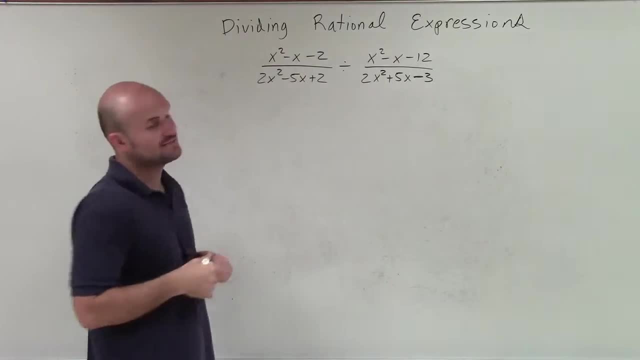 because it's a trinomial, so we know we're going to have to factor. So I have x squared minus x minus 2, and I need to determine. since my a is 1, I need to determine what two values multiply to give me negative 2, but then add to give me positive 1.. Well, 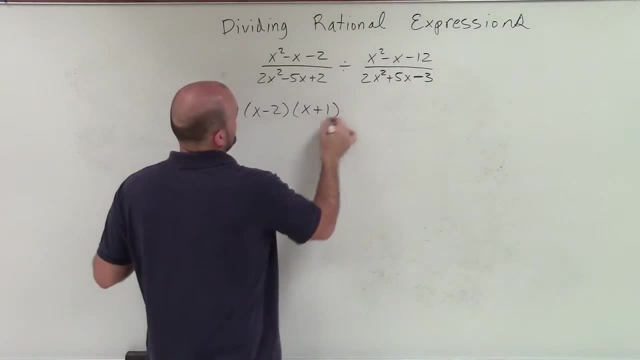 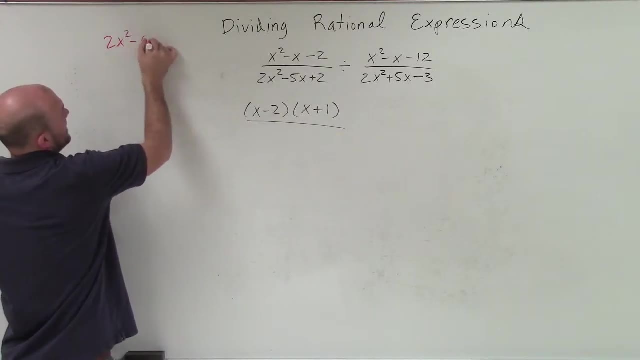 I can factor that to x minus 2 times x plus 1,. OK, That one wasn't so bad. This one's getting a little bit more difficult. So I have x plus 2,. all right, Now our a is not 1, so we can't just say what two numbers. 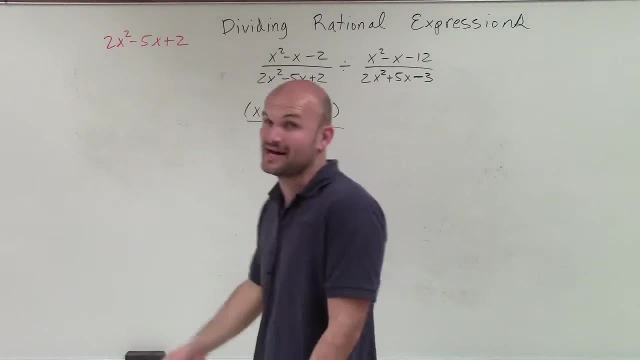 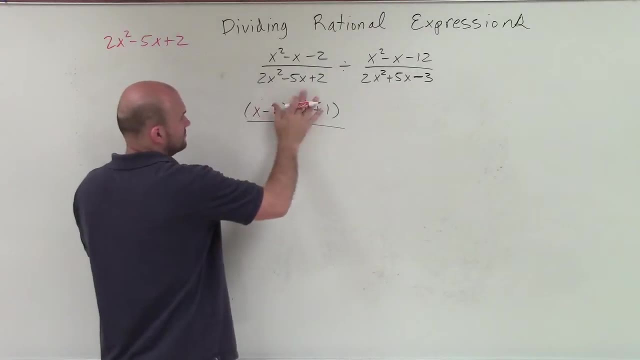 multiply to give me 2 and then add to give me negative 5.. It's a little bit more complicated than that. Remember, when we do FOIL we always say the first, so we're always going to multiply our first two terms. So we notice that our first two terms have to multiply to give us 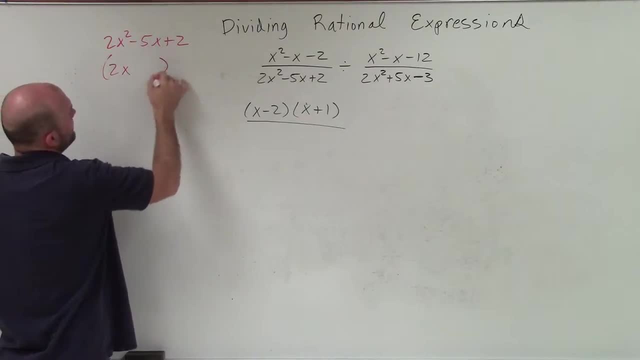 2x squared. So a lot of times what I like to do is just write out then: well, my first two terms then have to be 2x and x. They have to be. There's no other way unless we're going. 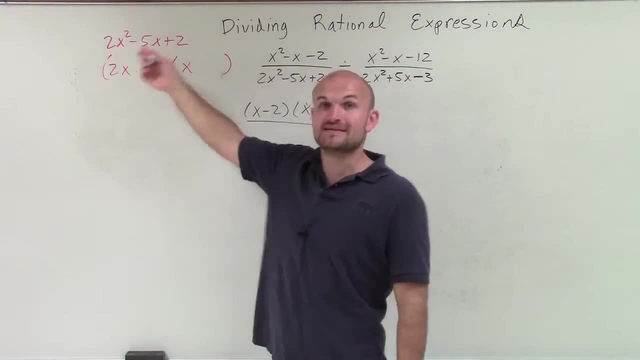 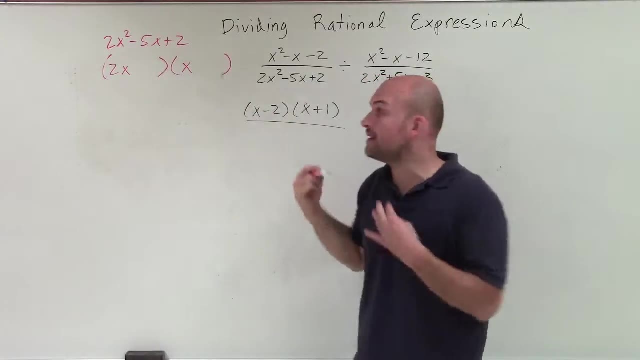 to get into fractions when we don't want to do that. Now we know our last two terms have to be positive 2. So it could either be 2 and 1 or negative 2 and negative 1.. And the way that we can determine which one it is is we. 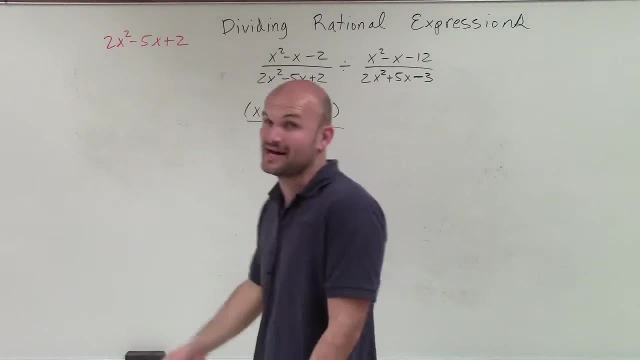 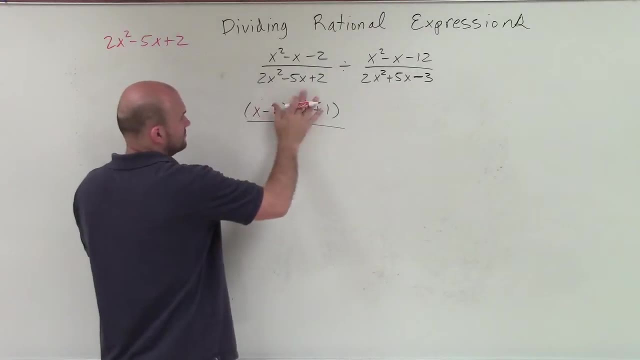 multiply to give me 2 and then add to give me negative 5.. It's a little bit more complicated than that. Remember, when we do FOIL we always say the first, so we're always going to multiply our first two terms. So we notice that our first two terms have to multiply to give us 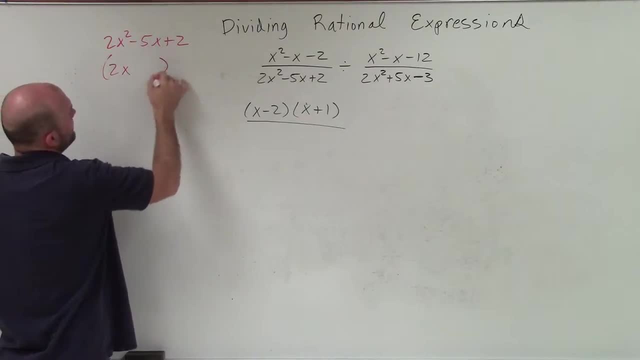 2x squared. So a lot of times what I like to do is just write out then: well, my first two terms then have to be 2x and x. They have to be. There's no other way unless we're going. 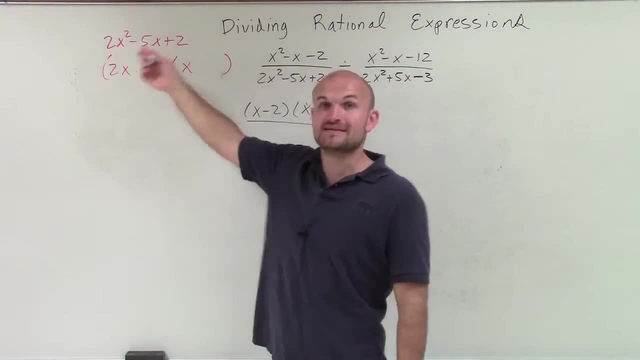 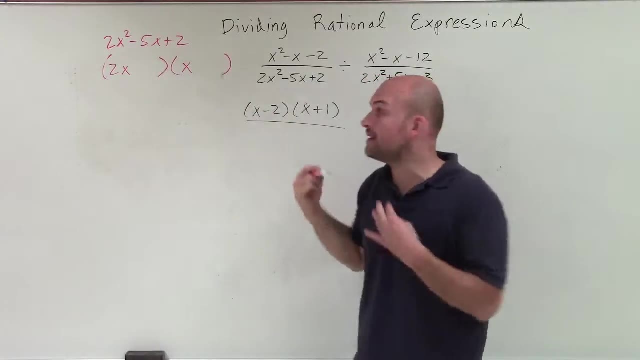 to get into fractions when we don't want to do that. Now we know our last two terms have to be positive 2. So it could either be 2 and 1 or negative 2 and negative 1.. And the way that we can determine which one it is is we. 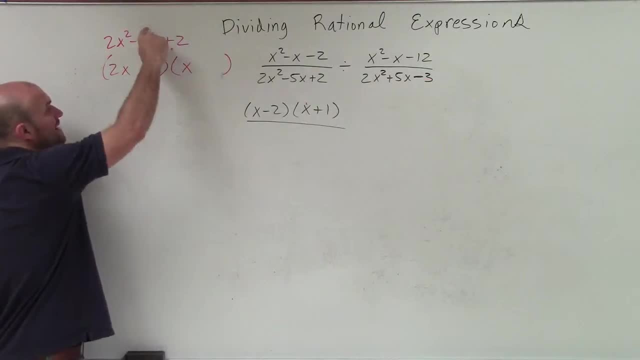 know that when we multiply our inner and our outer terms, they have to add up to negative 5, all right, So if I did, let's see here. we know well. first of all, we know they can't be positive because they all have to add up to a negative number. So our positive 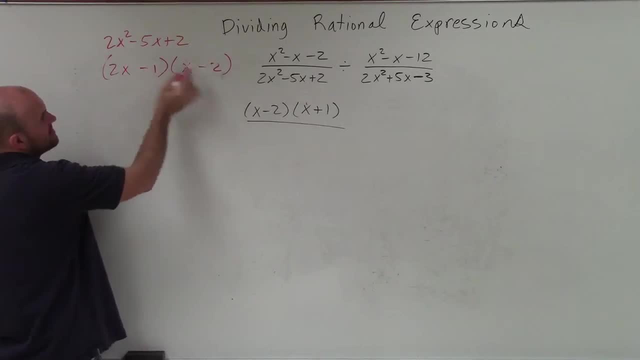 terms can't be right, So it has to be negative. Now, if I do negative 2x times negative 2,, that gives me a negative 4.. Plus x times negative 1,, that also gives me a negative 5,, which is my middle term. So therefore that's my correct factored form. So I'll just 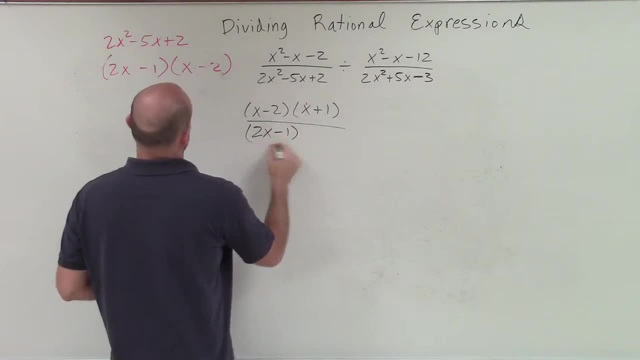 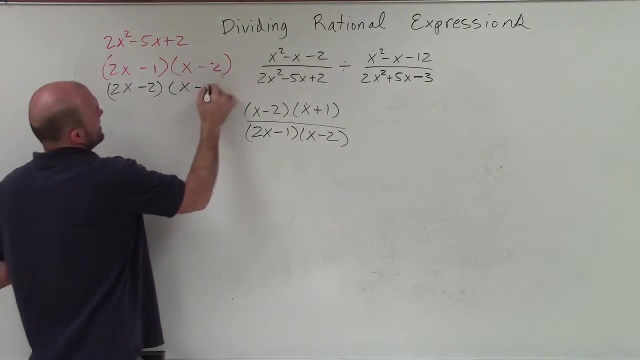 write that in there actually 2x minus 1, over x minus 2.. And the only other factored form we could have had was x minus 2, times x minus 1.. Now that doesn't work because 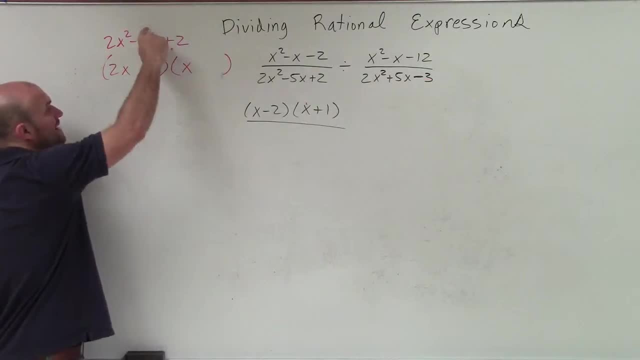 know that when we multiply our inner and our outer terms, they have to add up to negative 5, all right, So if I did, let's see here. we know well. first of all, we know they can't be positive because they all have to add up to a negative number. So our positive 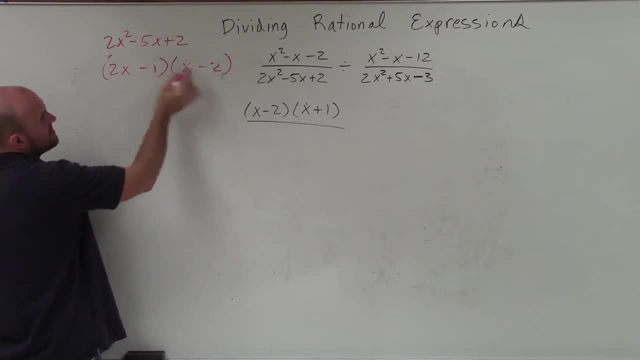 terms can't be right, so it has to be negative. Now, if I do negative 2x times negative 2, that gives me a negative 4 plus x times negative 1. That also gives me a negative 5,, which is my middle term. So therefore that's my correct factored form. So I'll just write: 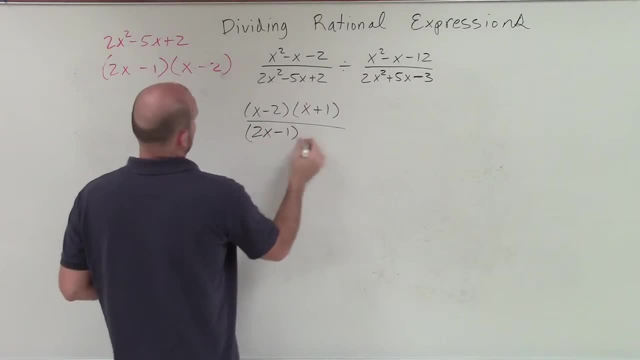 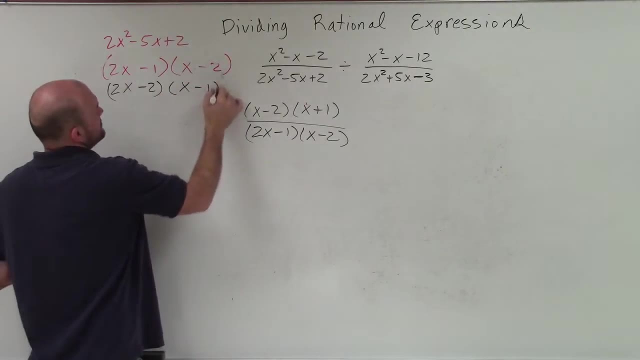 that in there actually 2x minus 1 over x minus 2.. And the only other factored form we could have had was x minus 2 times x minus 1.. And now that doesn't work because yes, x times x gives us 2x squared and negative 2 times 2. 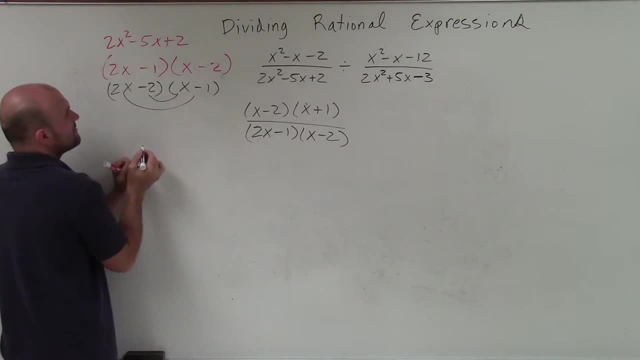 gives us a positive 2.. But when we add our outer and our inner 2x times negative, 1 is negative 4x. Negative 2 times x is negative 2x, which is a negative 4x. when you add them. 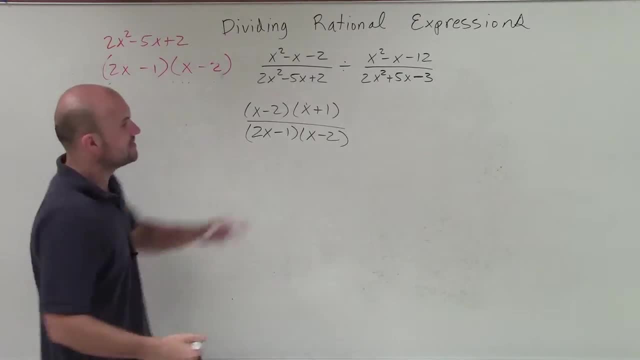 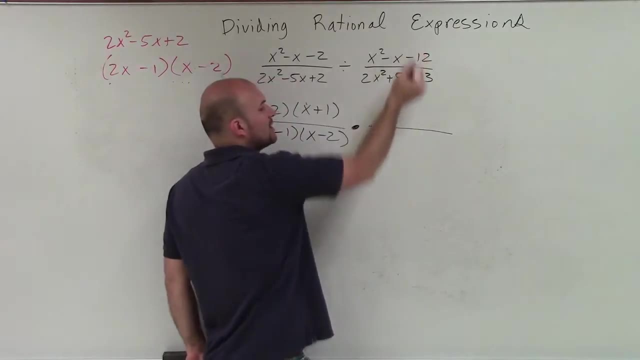 So that's why that does not work. So now we multiply and we reciprocate. So over here in my numerator is now going to become my denominator And I look at this. and since a is 1, I like factoring these problems now. 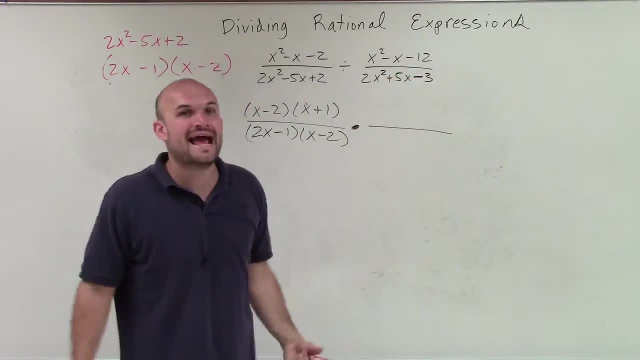 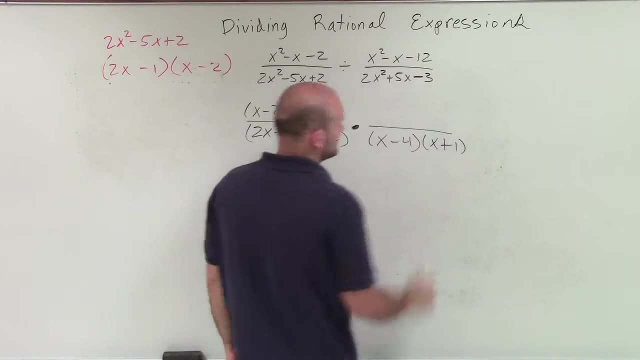 because you can just see what two numbers multiply to give me negative 12, but then add to give me a negative 1.. So therefore I can say that's going to be x minus 4 times x plus 1.. We like those problems. 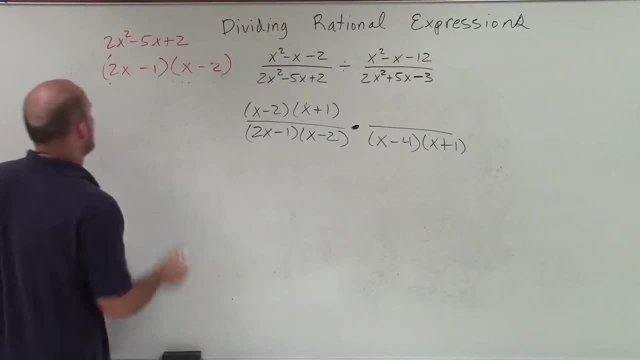 However, we have another one here. that's going to be when our a is equal to 2.. But that's OK. It's very similar to the one we just did. We know that my two factors have to start with 2x and x. 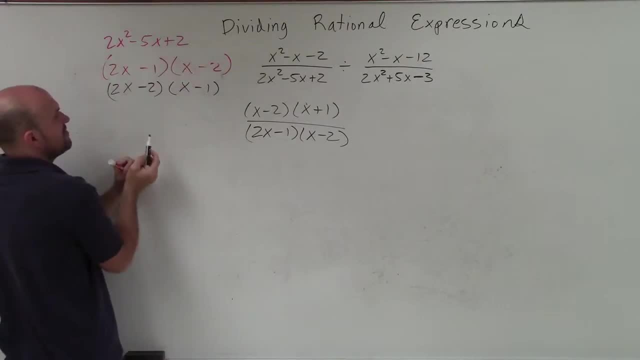 yeah, 2x times x gives us 2x minus 1.. I'm not sure if I got it right at all here, but 2x squared and negative 2 times 2 gives us a positive 2.. But when we add our outer and our inner, 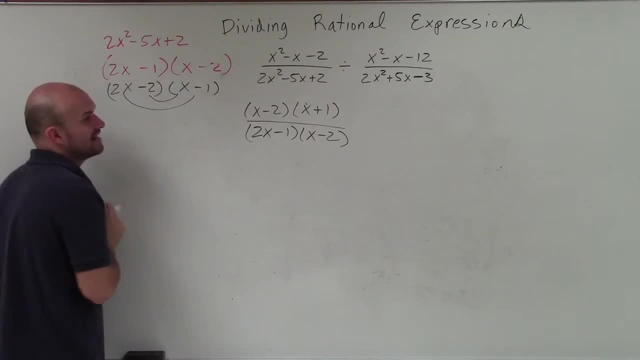 2x times negative. 1 is negative 4x. Negative 2 times x is negative 2x, which is a negative 4x when you add them. So that's why that does not work. So now we multiply and we reciprocate. 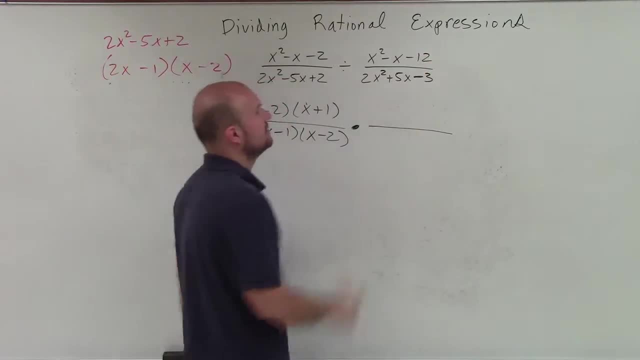 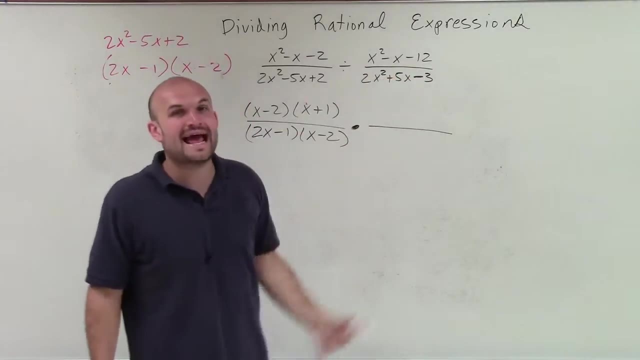 So over here in my numerator is now going to become my denominator And I look at this and since a is 1, I like factoring these problems now, because you can just see what two numbers multiply to give me negative 12, but then add to give me a negative 1.. 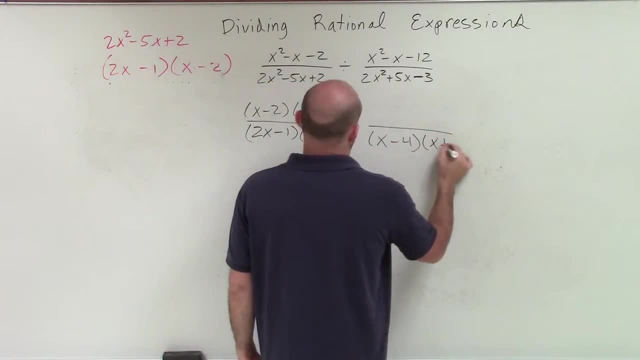 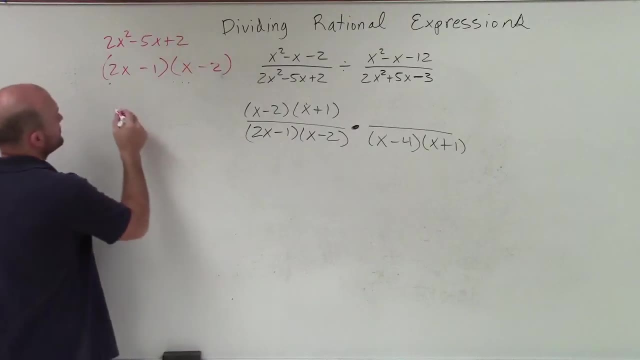 So therefore, I can say that's going to be x minus 4 times x plus 1.. We like those problems. However, we have another one here. that's going to be when our a is equal to 2.. But that's OK. 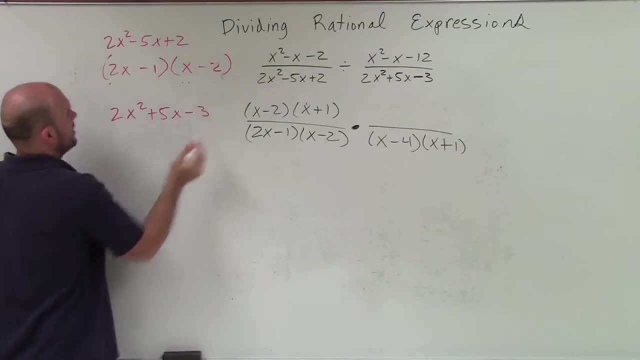 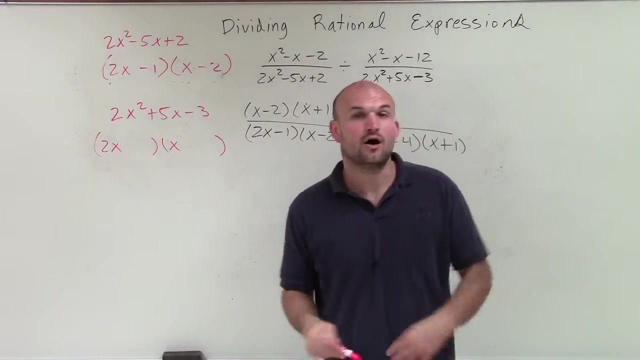 It's very similar to the one we just did. We know that my two factors have to start with 2x and x. Now my other two terms have to multiply to give me negative 3.. So the only two options I have is negative 3 and positive 1,. 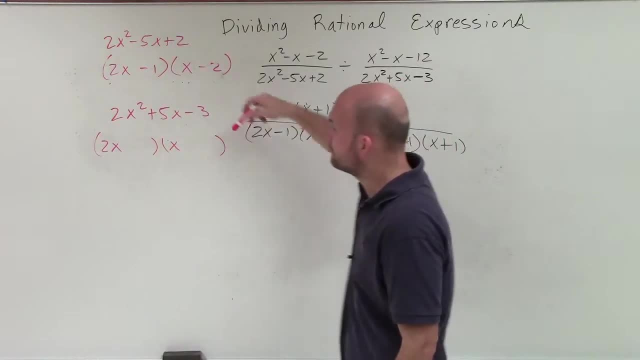 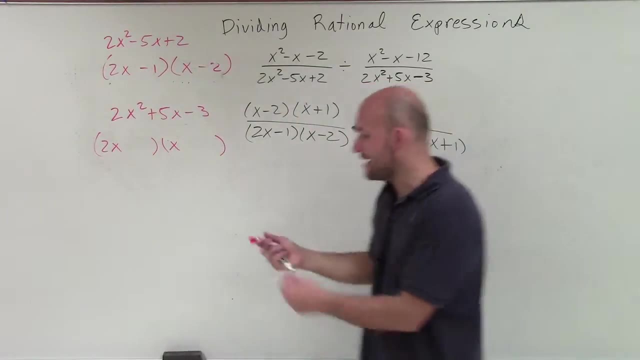 or positive 3 and negative 1.. And then we just need to determine, by adding our outer and our inner, what are going to add up to a positive 5x. So we know that the larger of the two multiplications has to be positive if our middle term 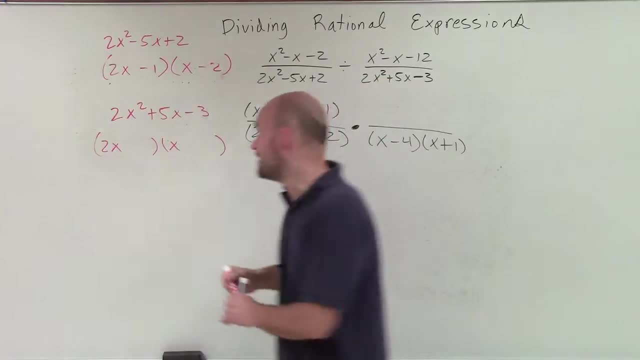 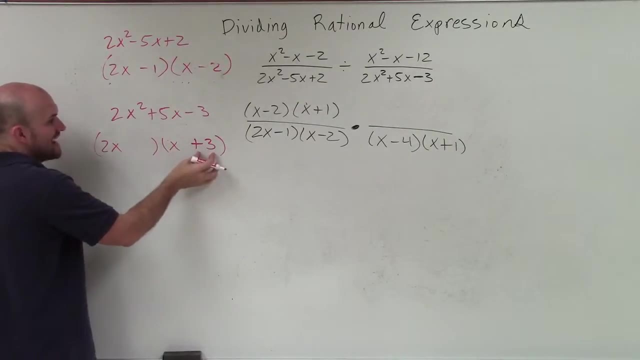 is going to add to a positive. So therefore, I know I'm going to have to multiply the 2x times my positive factor of 3, because, remember, I want to add them to make them positive. So I don't want to have 2x times negative 3.. 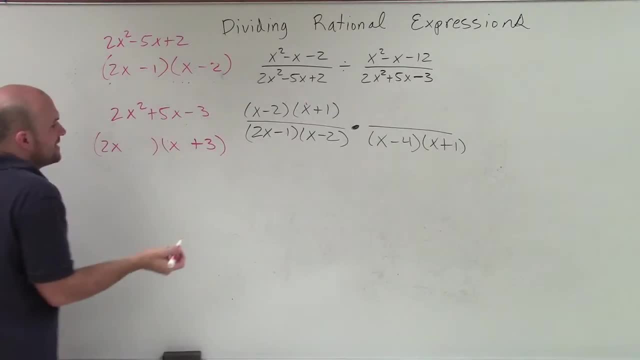 That would give me negative 6,, 6x right, And that means I'm going to have a negative problem, negative number. I want it to be positive. So if that's positive, then that means that one has to be negative. 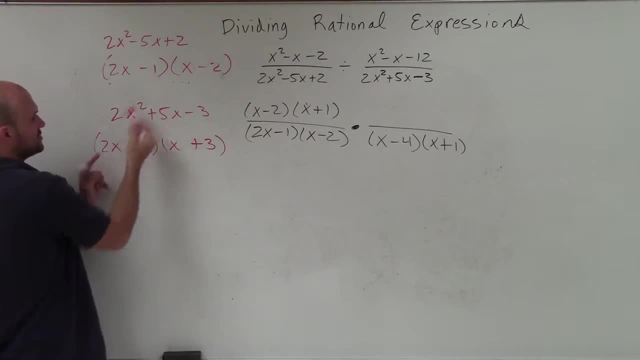 And we can just double check that Again. that goes to negative 3.. That goes to 2x squared. When I combine my inner and my outer, 2x times 3 is 6x. Negative x times x is negative 1x. 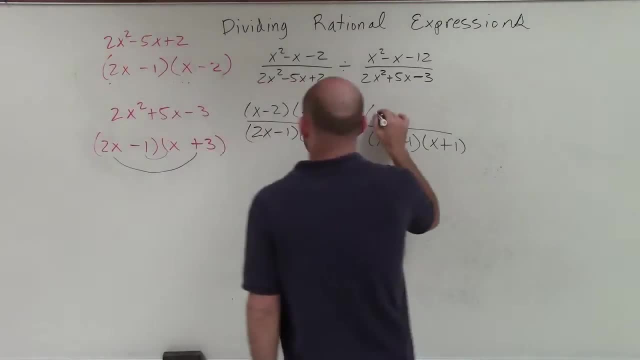 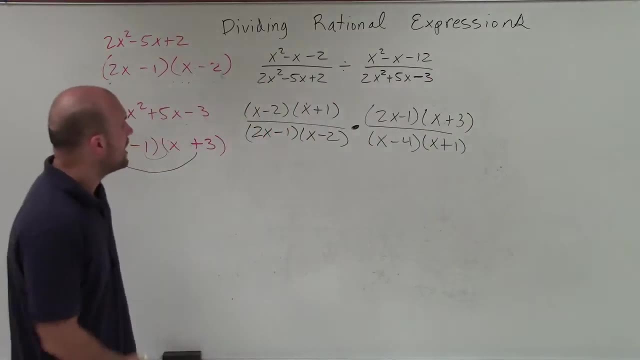 6x minus x is positive 5x. So now let's write these in there, So I have 2x minus 1 over an x plus 3.. OK, so now what we can take a look at this is: oh. 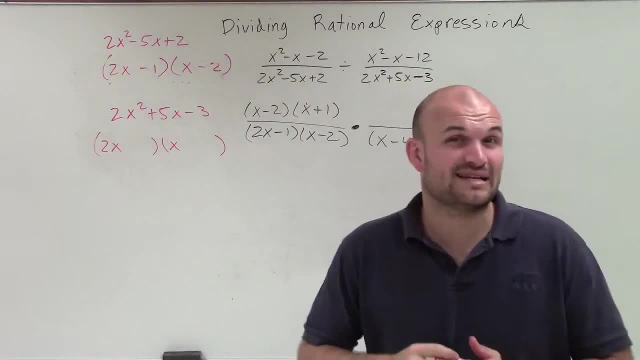 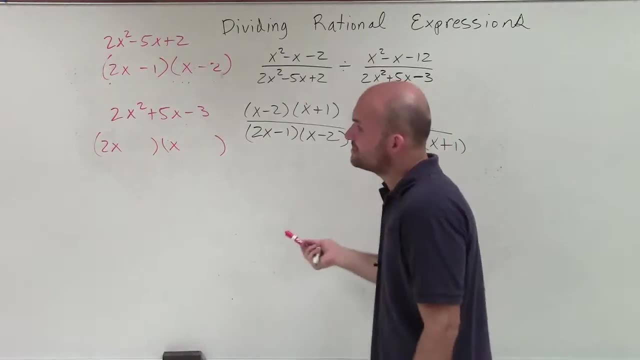 Now my other two terms have to multiply to give me negative 3.. So the only two options I have is negative 3 and positive 1, or positive 3 and negative 1.. And then we just need to determine by adding our outer. 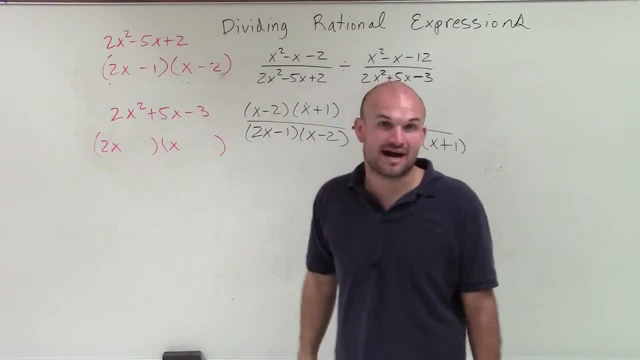 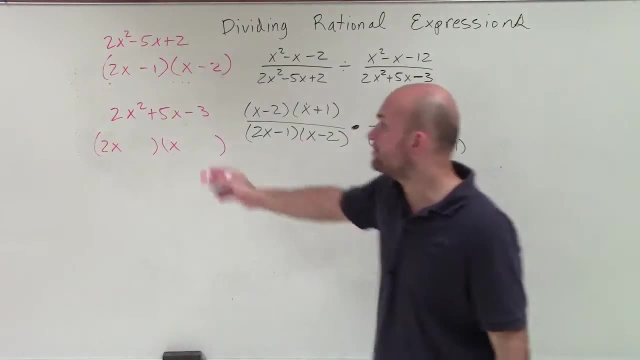 and our inner what are going to add up to a positive 5x. So we know that the larger of the two multiplications has to be positive if our middle term is going to add to a positive. So therefore, I know I'm going to have to multiply the 2x times. 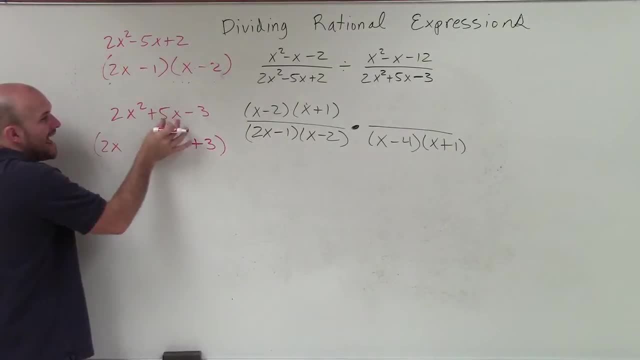 my positive factor And I want to get a negative 3.. And the negative 3 is going to give me a negative 3.. So I'm going to add 2x to the negative 3.. And then I want to add negative 3 to the negative 3.. 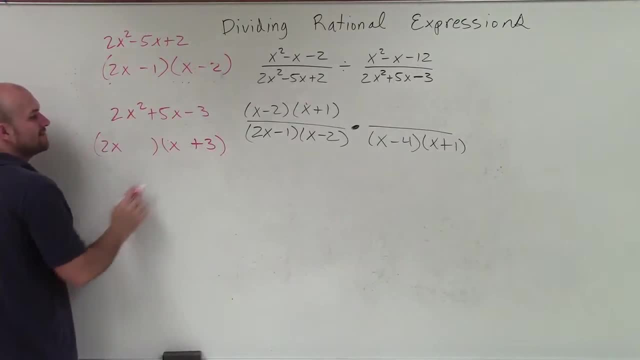 Because, remember, I want to add them to make them positive, So I don't want to have 2x times negative 3. That would give me negative 6. 6x right, And that means I'm going to have a negative problem. 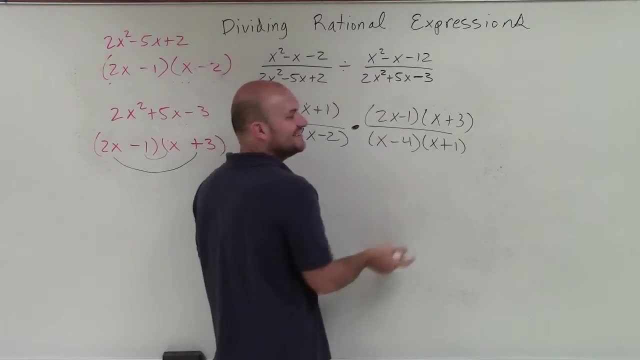 that is definitely not right. Negative 4, sorry, What two numbers multiply to give you negative 12, but then add to give you negative 1? Well, it's going to be x minus 4 and x plus 3.. Sorry about that. 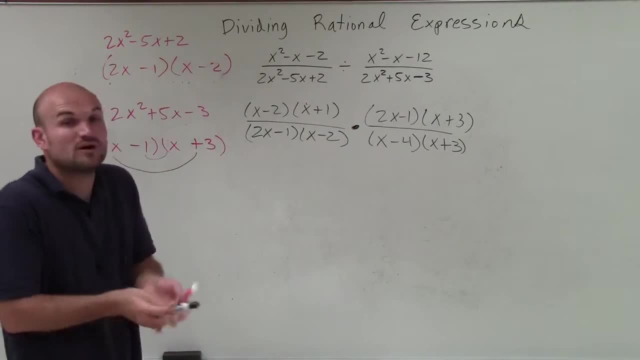 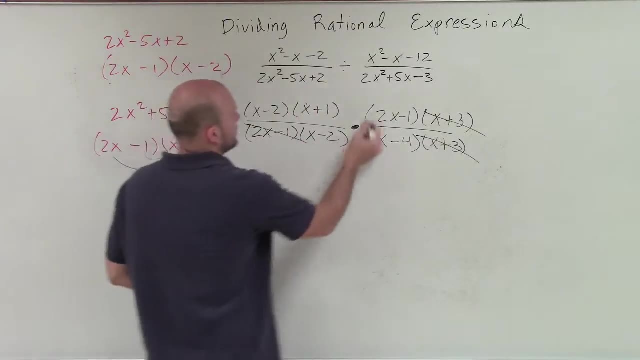 OK, so now we just need to take our terms and see which values can be divided by the terms in the denominator. Well, that divides into 1.. Those two divide into 1.. And those divide into 1, leaving me with my final answer of x plus 1 divided by x minus 4..